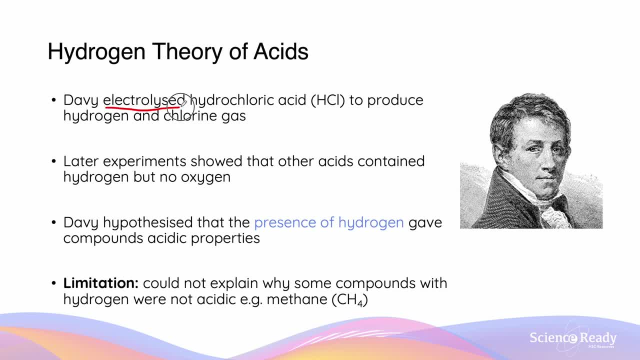 and he did this through using the electrolysis chemical separation theory on hydrochloric acid in order to produce hydrogen and chlorine gas. So what later experiments, including this one, showed was that there were other acids which contained hydrogen, but they did not contain oxygen. 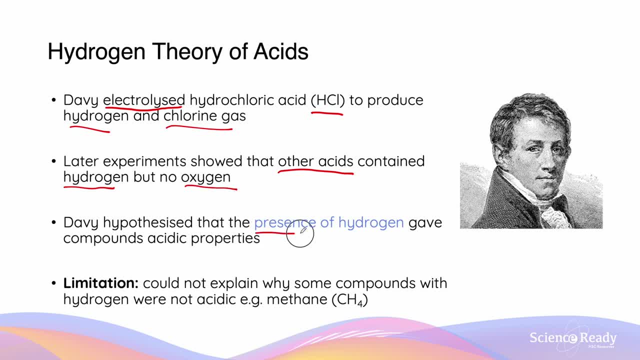 As a result of this, Davy hypothesized that it was actually the presence of hydrogen which gives compounds their acidic properties. Again, this theory was limited, as the theory did not explain why some compounds that had hydrogen were not acidic, For example Methane. 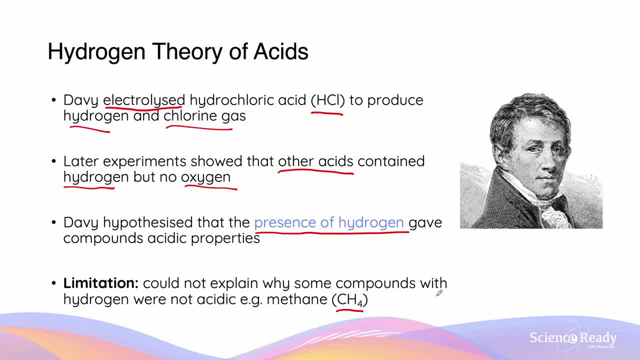 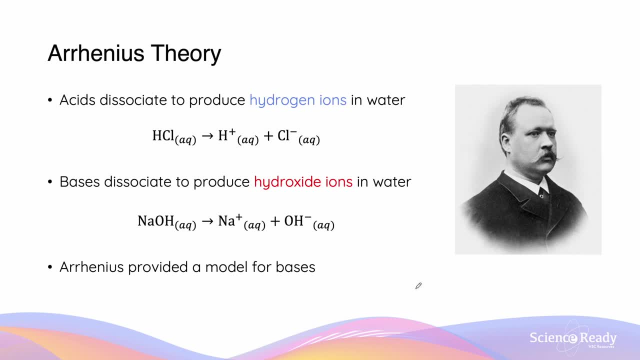 contains 4 hydrogen, but it is not an acidic compound. The Arrhenius Theory is one of two main theories which are central to the acids and bases module. The Swedish scientist Farntey Arrhenius gave an example of the meaning for the acompanza. 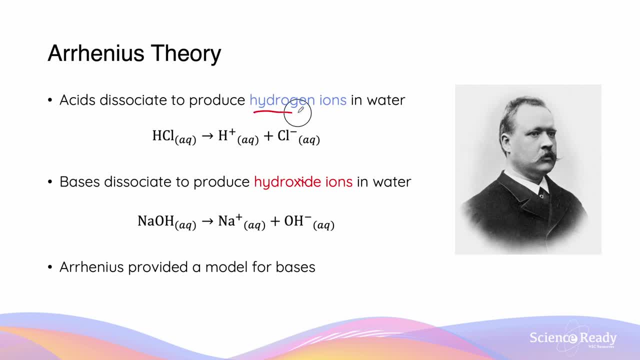 described acids as being able to produce hydrogen ions when dissociated in water. However, bases he described were ones that produced hydroxide ions when dissociated in water. At the top we can see we have a hydrochloric acid, HCl, which dissociates to produce the H plus ion and the Cl minus ion in water. 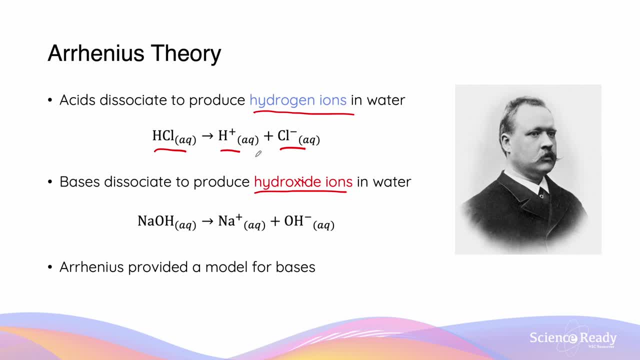 Because H plus is being produced in water, HCl is described as being an Arrhenius acid. Similarly, with NaOH sodium hydroxide, we get the production of the Na plus sodium ion and the OH minus hydroxide ion, and therefore this NaOH can be described as being an Arrhenius base, The Arrhenius 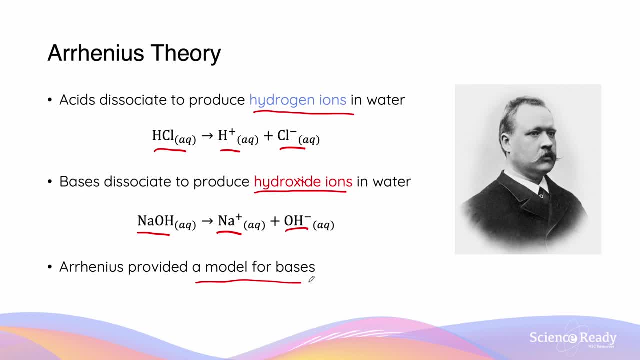 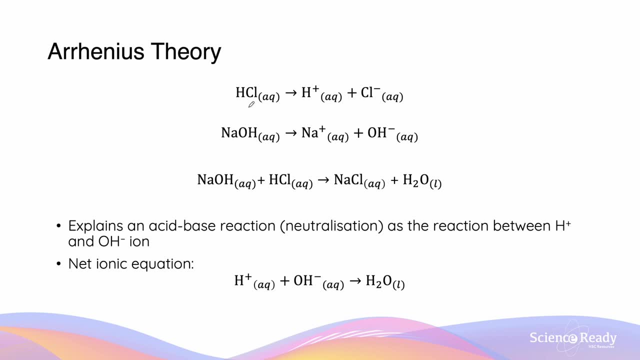 model was actually the first model which provided a model that included ones for bases. We may have explored the Arrhenius theory briefly in stage 5.. As we can see, we earlier talked about HCl dissociation into H plus and Cl minus, and NaOH dissociating into Na plus and OH minus. 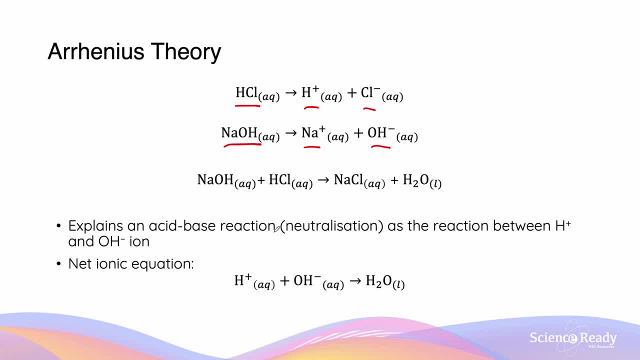 The Arrhenius theory is effective in that it explains how acid-base reactions, also known as neutralization reactions, help to form water to the reaction of the hydrogen ion and the hydroxide ion which is produced And we have the net ion equation: H plus plus, OH minus forms H2O liquid. We can see the. 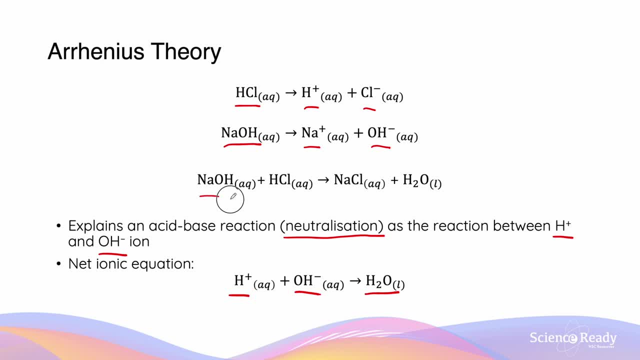 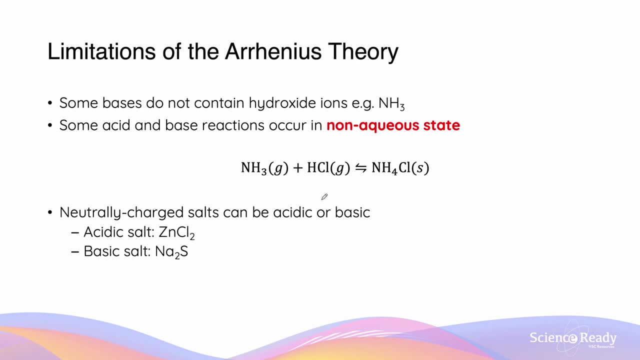 formation of water from the neutralization reaction between sodium hydroxide and HCl hydrochloric acid. The Arrhenius theory, however, also has its limitations. The Arrhenius theory does not explain how some bases like NH3 do not contain any hydroxide ions. It also does not explain how some acid-base reactions 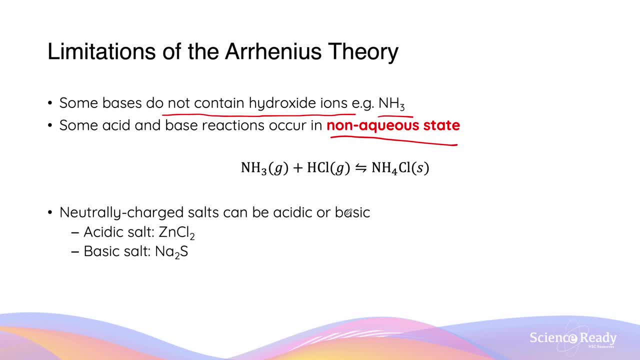 can occur in the non-aqueous state, meaning that reactions can occur outside of water. Here we have an example of an acid-base reaction which occurs in the non-aqueous state. Ammonia NH3 reacts with hydrogen chloride, which is hydrochloric acid in the gaseous state, in order to form the ammonium chloride. 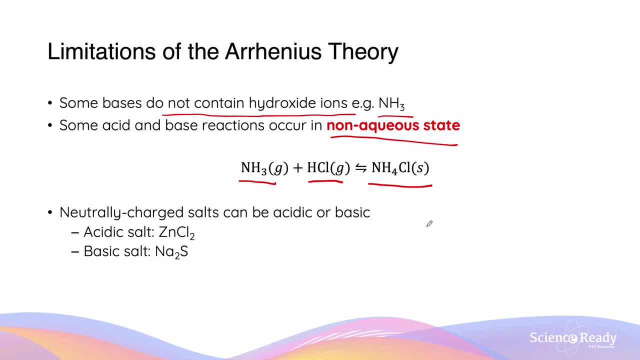 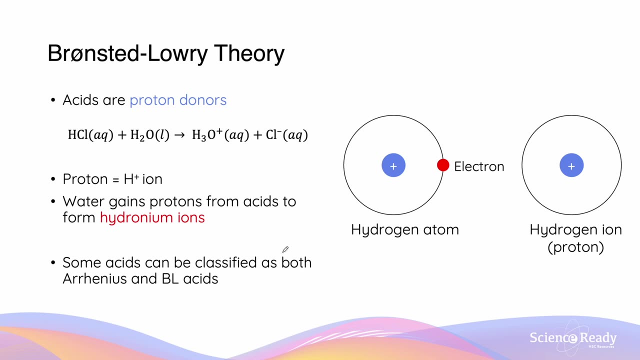 salt. The Arrhenius theory also does not help to explain how neutrally charged salts such as zinc chloride or sodium sulfide can be acidic or basic. So the limitations of the Arrhenius theory, which we previously discussed, are overcome by the Bronsted-Lowry theory. The Bronsted-Lowry theory states that the 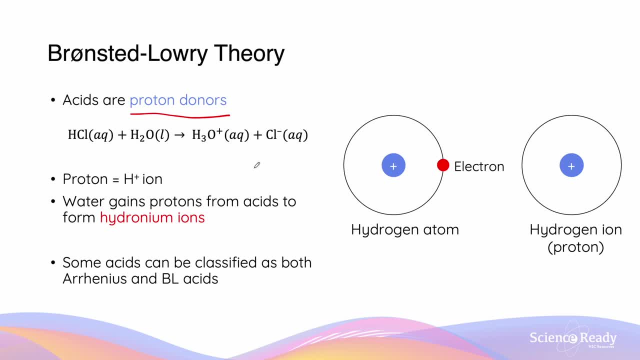 acids are proton donors. We know that the hydrogen ion is simply a proton, as the hydrogens contain one proton and one electron, and the formation of a hydrogen cation comes from the loss of its singleton electron. If we look at this equation below here, we can see that hydrogen chloride or hydrochloric acid 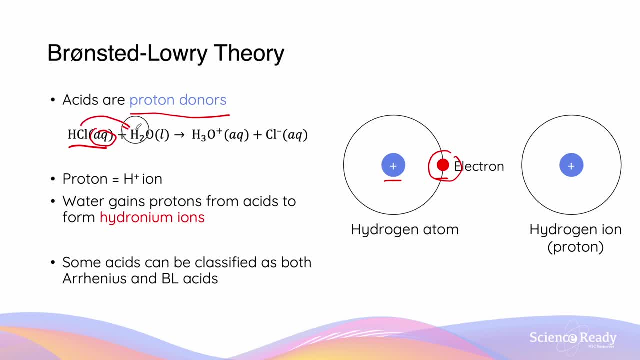 in this case, because it's aqueous, donates its proton to H2O in order to form H3O and H3O2, which is the hydronium ion, and Cl- which is a chlorine anion. Since the hydrochloric acid engaged in the donation of a proton, it can be. 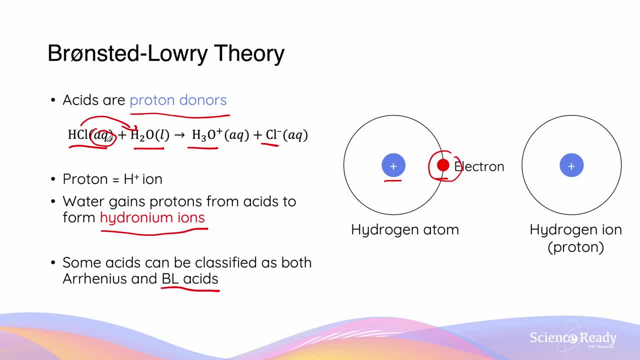 classified as a Bronsted-Lowry acid Because the hydrochloric acid also dissociated in the water to produce an H plus ion. it can also be classified as an Arrhenius acid, and some acids can be classified as both Arrhenius and 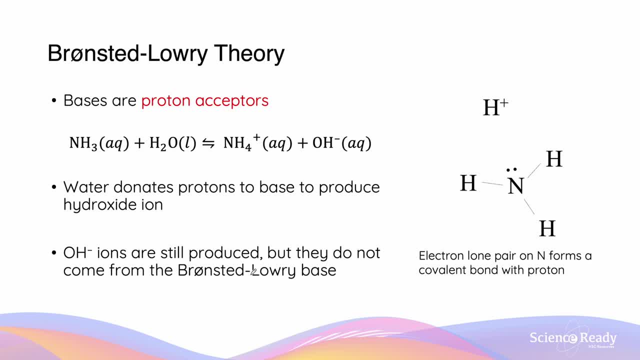 Bronsted-Lowry acids. Conversely, the Bronsted-Lowry theory also states that the hydrochloric acid is a proton, and it is a proton that is a proton, In this case NH3- reacts with H2O to form NH4 plus and OH minus. The ammonium ion is 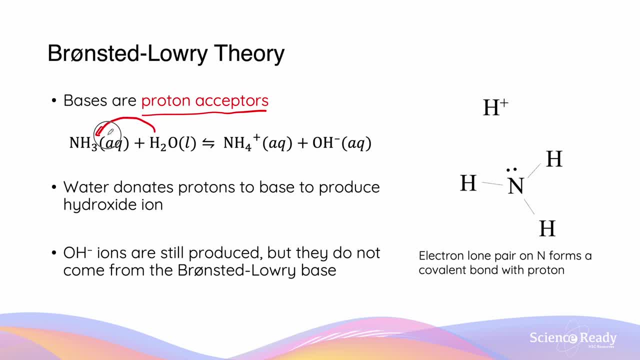 actually formed from the acceptance of a proton which is donated from H2O. The donation of the proton from the water molecule is actually what leads to the formation of the hydroxide ion in water, according to the Bronsted-Lowry theory. So in the Bronsted-Lowry theory, hydroxide ions are still being produced. 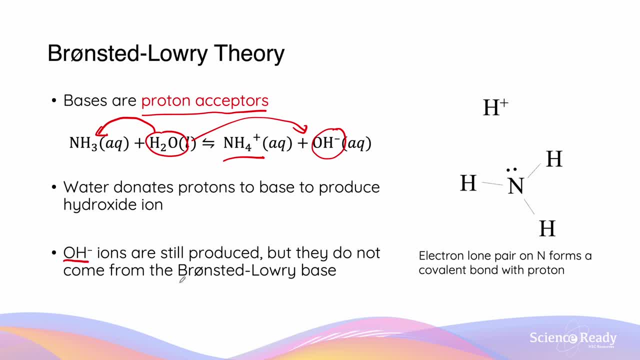 by bases. However, they do not come from the dissociation of the Bronsted-Lowry base. The reason why the NH3 is able to react in the water with the H plus ion is because there is the existence of a lone pair on the nitrogen in order to 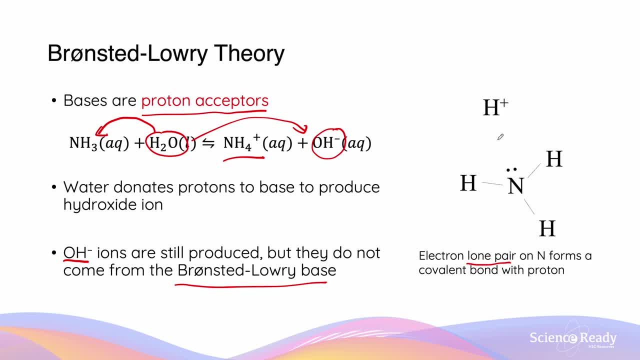 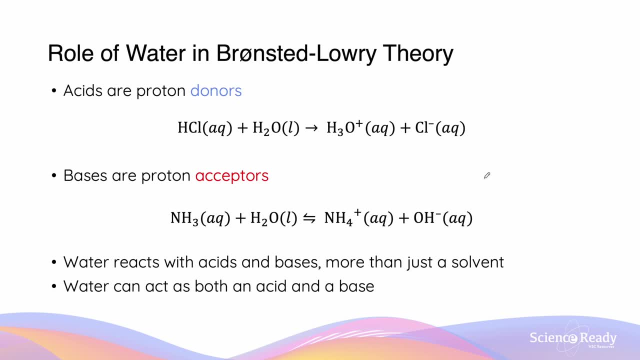 form a covalent bond with the proton which is donated from H2O. Bronsted-Lowry theory also explains conjugate pairing. If we study these two equations below, we can see what kind of role water plays in a reaction between a Bronsted-Lowry acid. 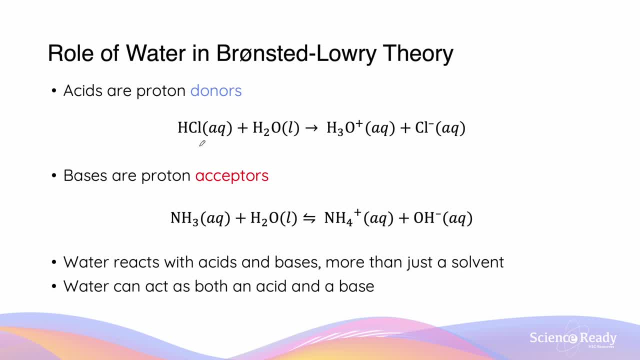 and a Bronsted-Lowry base, We've established that hydrochloric acid is an acid because it donates its proton. We know that ammonia is a base because it accepts a proton. In the top case, water is actually accepting a proton in order. 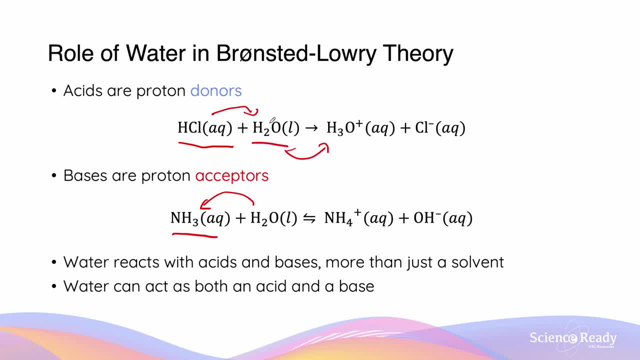 to form the hydronium ion. So it's acting as a proton acceptor and therefore in the top equation is acting as a base. In the bottom equation, H2O is actually donating its proton. therefore it is acting as a Bronsted-Lowry acid. This characteristic 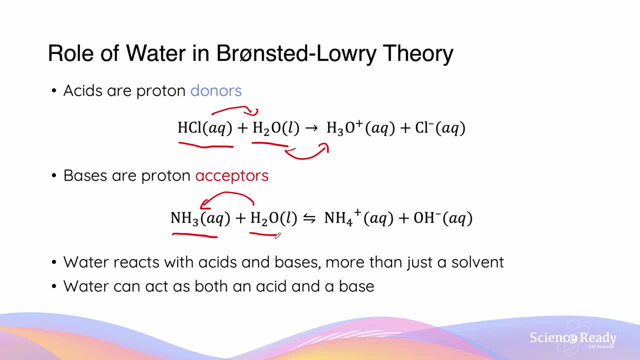 of water being able to act as both an acid and a base and the role which it plays in reactions is different in the Bronsted-Lowry theory than the Arrhenius theory, where water is just a solvent. Here is a demonstration of how the reaction between a Bronsted-Lowry 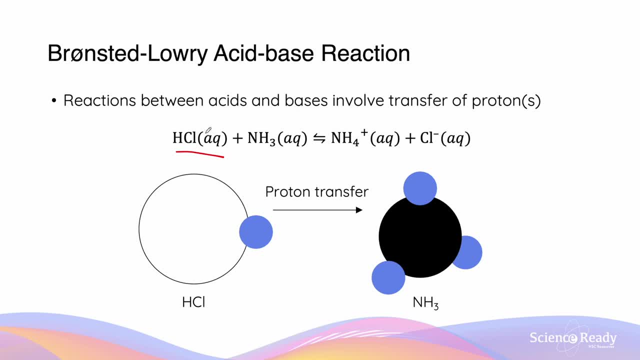 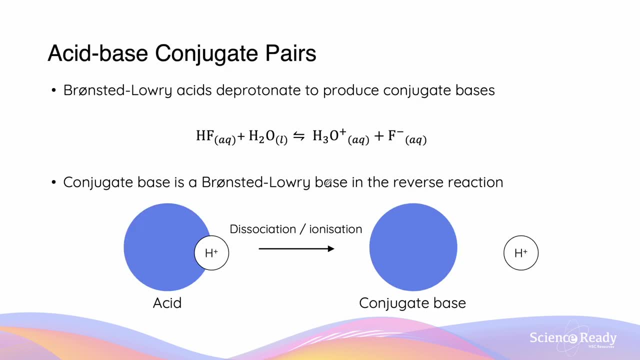 acid. hydrochloric acid donates its proton to react with a Bronsted-Lowry base, ammonia. Bronsted-Lowry theory also helps to explain conjugate pairing. The Bronsted-Lowry acid deprotonates to produce a conjugate base, In this first case hydrogen fluoride. also. 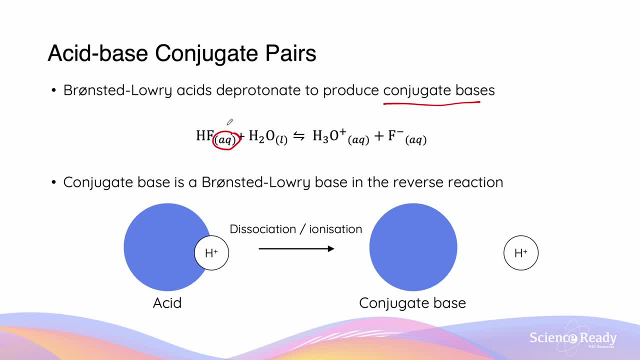 known as hydrochloric acid. in its aqueous state, donates its proton to water to create the fluoride ion, which is its conjugate base. This is called the conjugate base because it has the ability to reform the hydrochloric acid by accepting a proton which is donated. 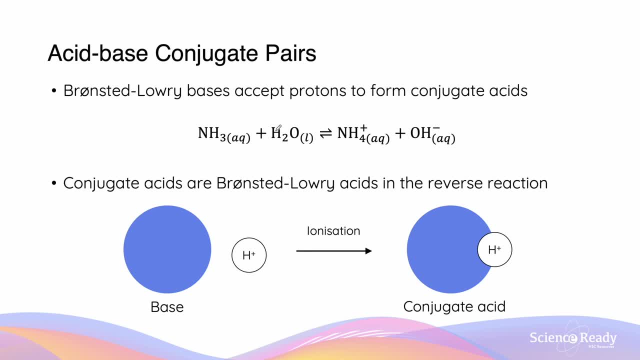 from the hydronium ion. Similarly, in the opposite case, the Bronsted-Lowry base will accept protons to form a conjugate acid. In this scenario, ammonia forms ammonium through the acceptance of a proton that's donated from H2O. This ammonium is then able to donate its own proton to the hydroxide. 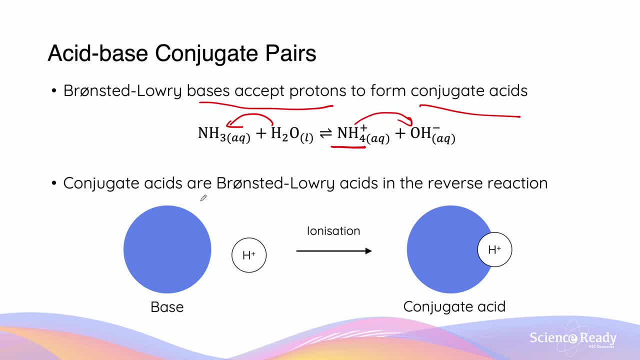 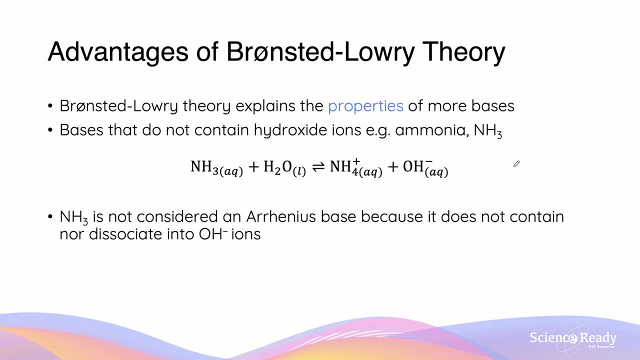 ion to reform water. So conjugate acids are Bronsted-Lowry acids. in the reverse reaction, Bronsted-Lowry theory maintains the same principle. The Bronsted-Lowry theory maintains the same principle but uses a few advantages over the Arrhenius theory. It helps to explain. 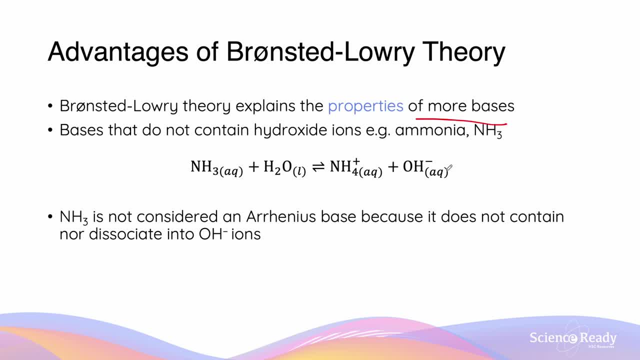 the properties of more bases, including how some bases do not need to contain hydroxide ions, such as ammonia, And we discussed earlier how the hydroxide ion, which is still formed in the Bronsted-Lowry theory, does not come from the dissociation of the base, but actually 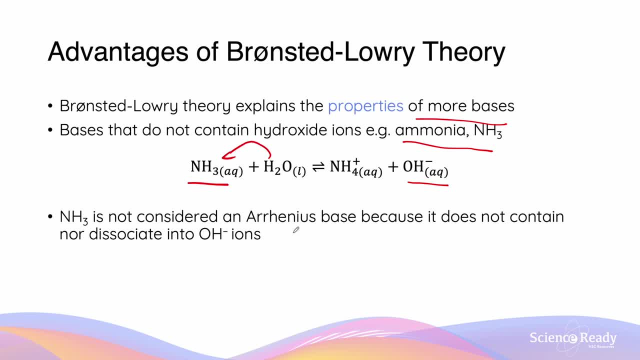 comes from the donation of a proton from the water. The example that we commonly use is ammonia, which is not considered an Arrhenius base, but that is the same principle we commonly use because it does not contain or dissociate into hydroxide ions, but is considered a Bronsted-Lowry. 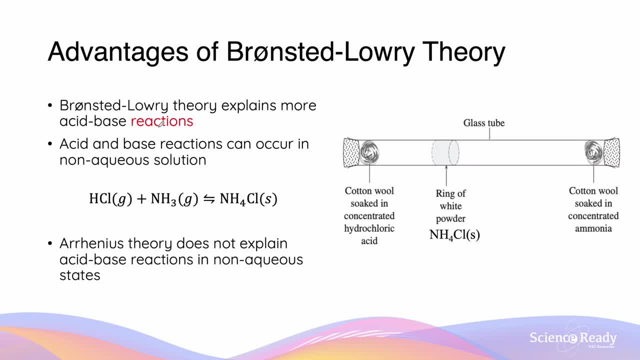 base. The Bronsted-Lowry theory also explains more acid-base reactions, also known as neutralisation reactions. In particular, the Bronsted-Lowry theory explains how acid-base reactions can occur in a non-aqueous solution. Here we have hydrogen chloride in the gaseous state, reacting with 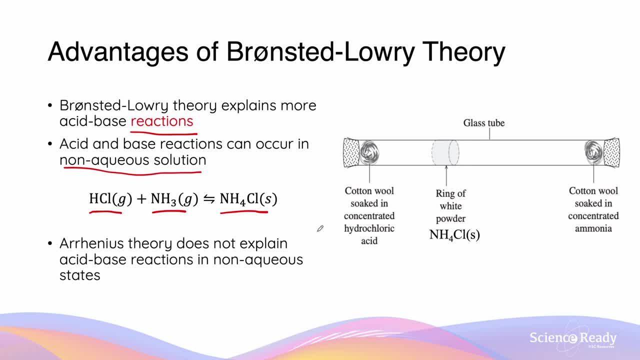 ammonia to form ammonium chloride. We have an example of how this reaction works on our diagram on the right hand side, where we have cotton balls soaked in concentrated hydrochloric acid and cotton balls soaked in concentrated ammonia. In this case, the acid-base reaction occurs. 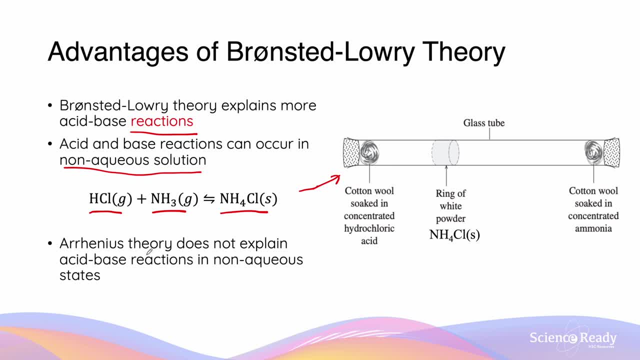 from the fumes which are produced from the soaked cotton balls. The inability for the Arrhenius theory to explain acid-base reactions in a non-aqueous state is actually one of its greatest limitations. So other advantages of the Bronsted-Lowry theory: Well, the Bronsted-Lowry theory also. 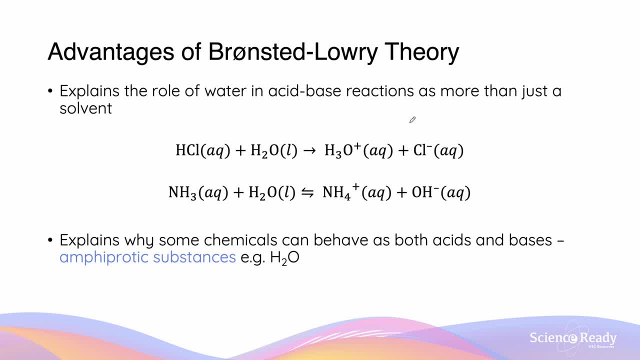 explains what the role of water is in the acid-base reactions as more than just a solvent. We previously looked at these equations where we had water acting as a base and water acting as an acid. So the Bronsted-Lowry theory explains why some chemicals such as water,